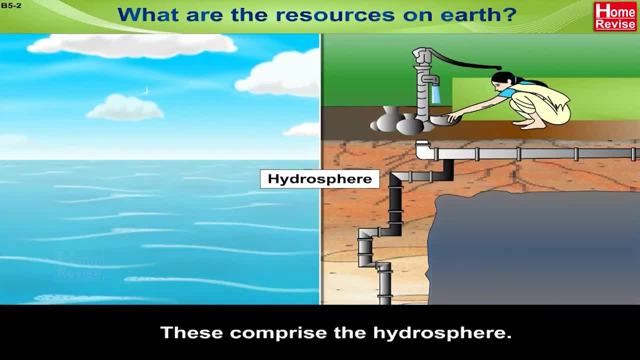 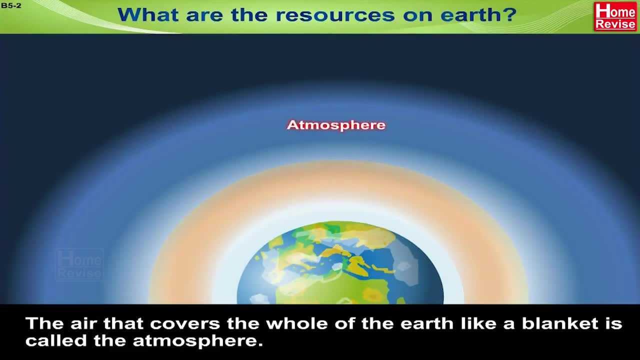 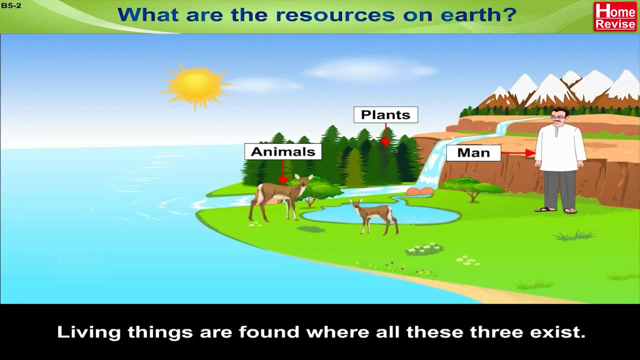 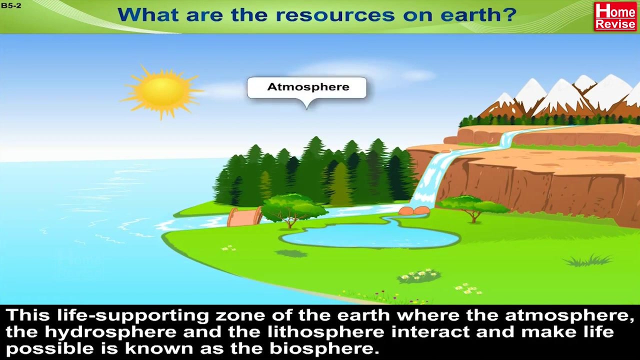 These comprise the hydrosphere. The air that covers the whole of the Earth like a blanket is called the atmosphere. Now, living things are found where all these three exist, This life-supporting zone of the Earth where the atmosphere, the hydrosphere and the lithosphere. 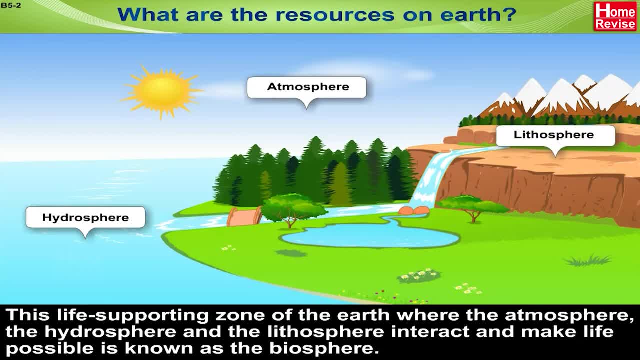 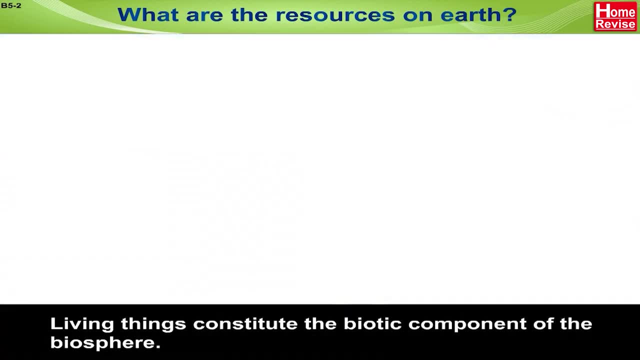 interact is called the atmosphere sandbox: Energy and water, making us the objects of the earth. right, It is called the water- planet. do you know what is called this atmosphere? Well, it is the biosphere. насRAC, Rising sea level. 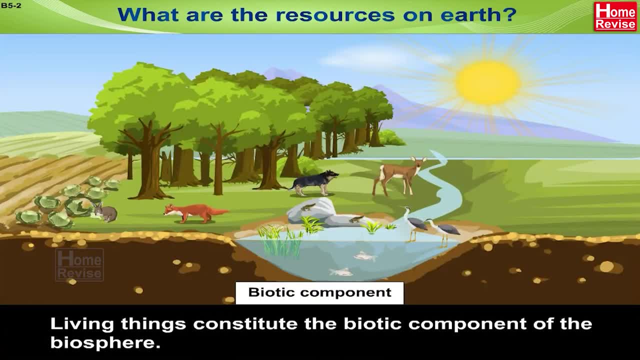 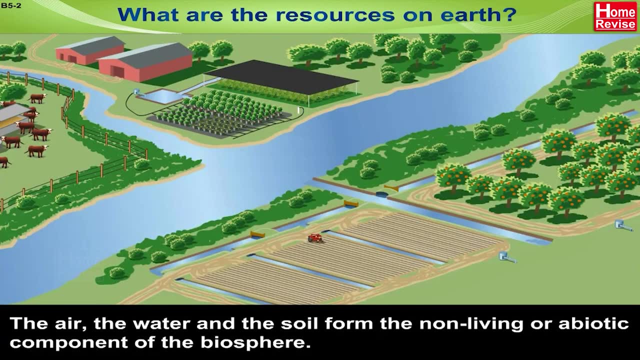 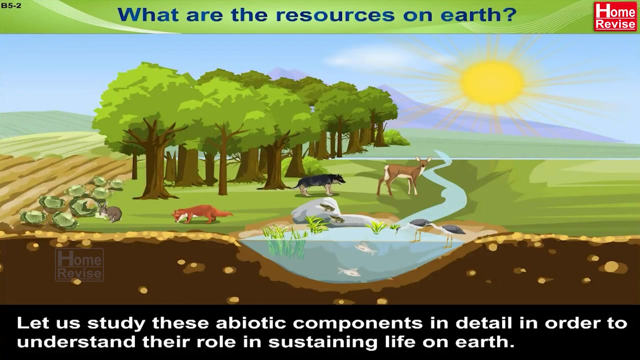 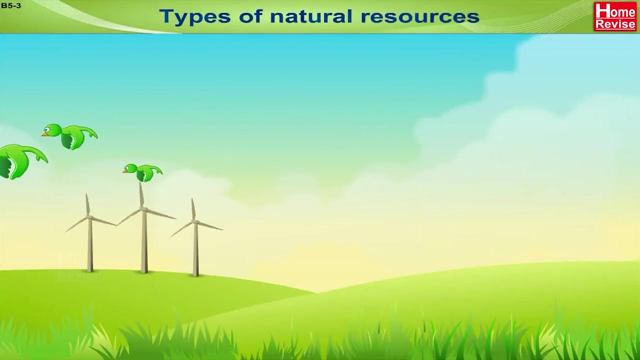 Living things constitute the biotic component of the biosphere. Res collateral air, water and soil form the non-living or abiotic component of the biosphere earth round. invite root these abiotic components in detail in order to understand their role in sustaining life on earth. types of natural resources. renewable resources. 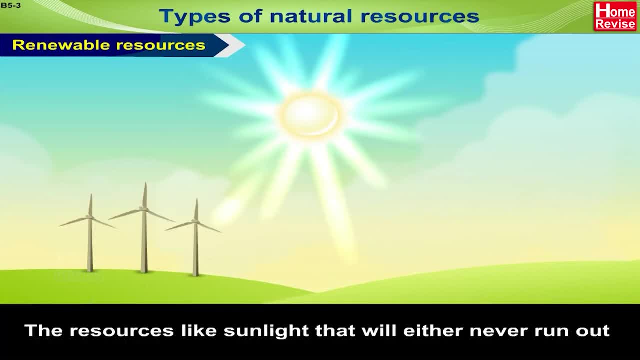 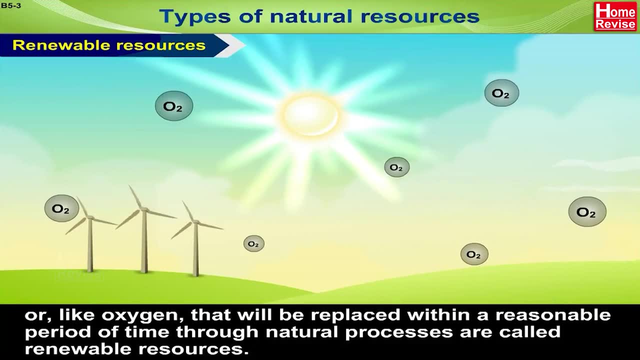 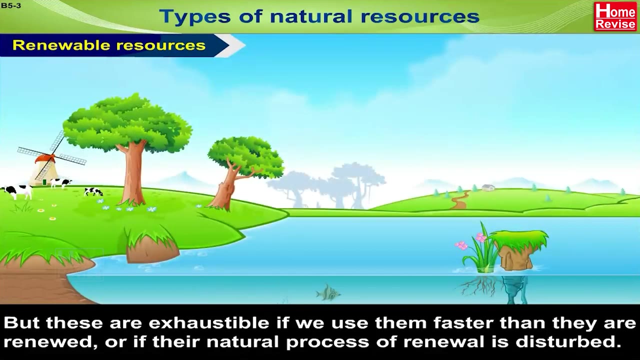 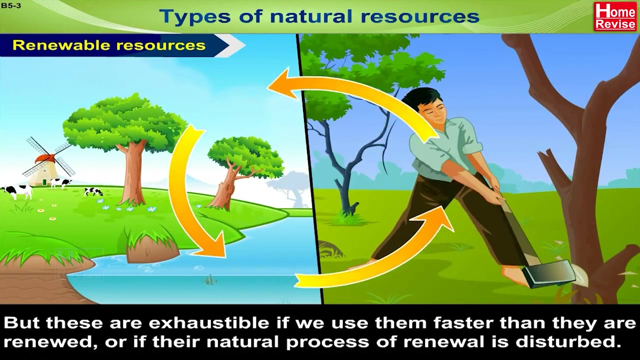 the resources like sunlight that will either never run out, or like oxygen that will be replaced within a reasonable period of time through natural processes, are called renewable resources, but these are also exhaustive will if we use them faster than they are renewed or if the natural process of renewal is disturbed. 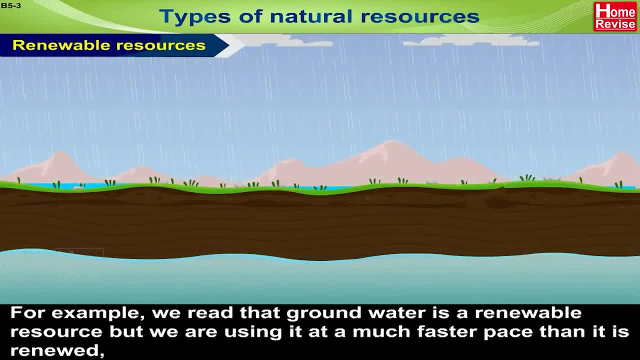 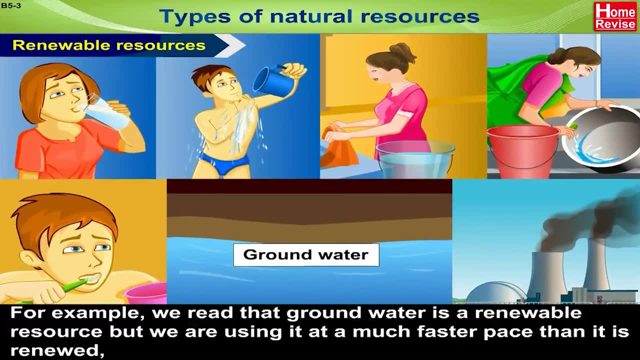 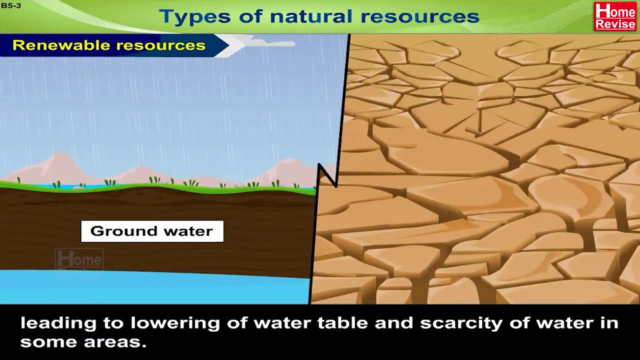 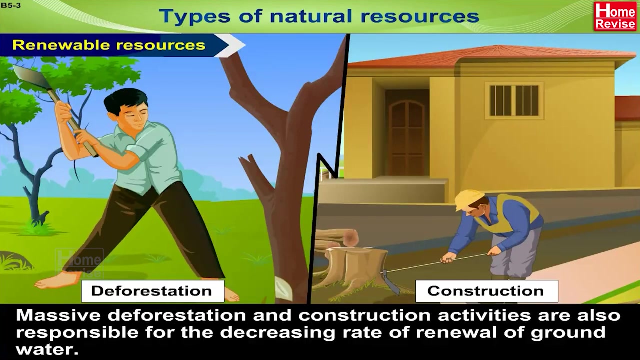 for example, we read that groundwater is a renewable resource, but we are using it at a much faster pace than it is renewed, leading to lowering of water table and scarcity of water in some areas. Massive deforestation and construction activities are also responsible for the decreasing rate of renewal of groundwater. 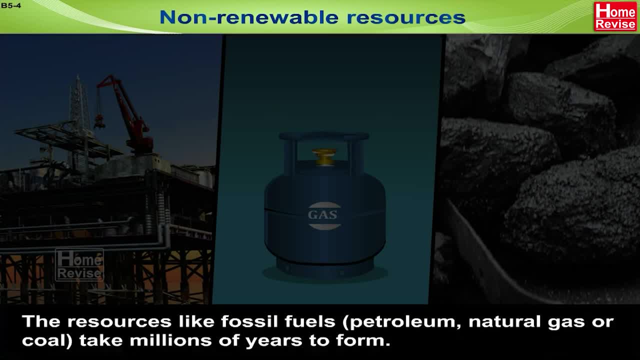 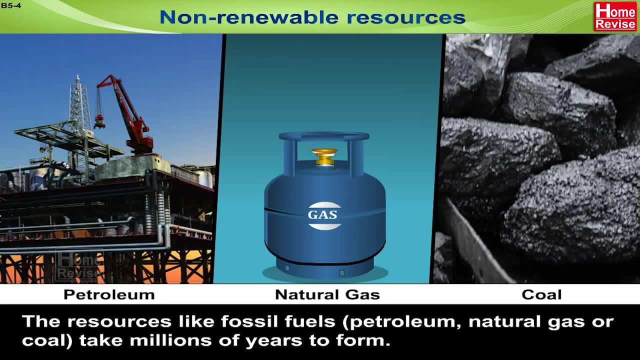 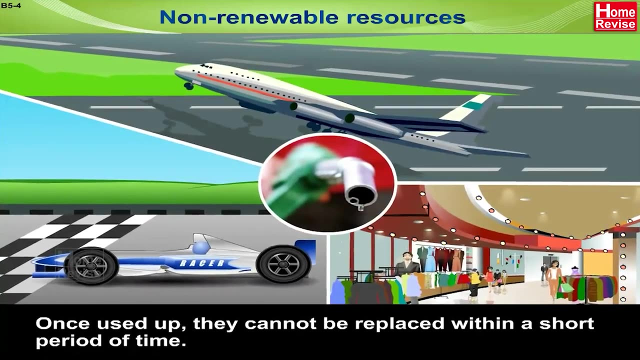 Non-renewable resources. The resources, like fossil fuels, which are petroleum, natural gas or coal, take millions of years to form. Once used up, they cannot be replaced within a short period of time. These are called non-renewable resources. 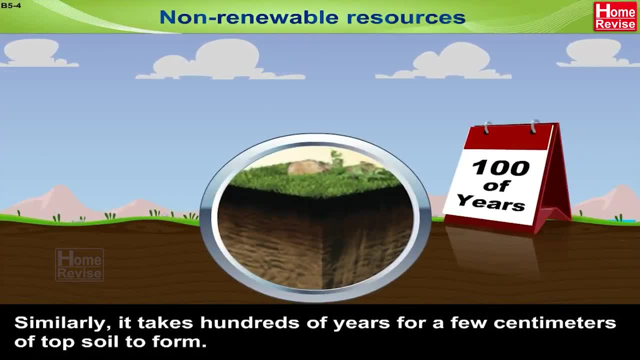 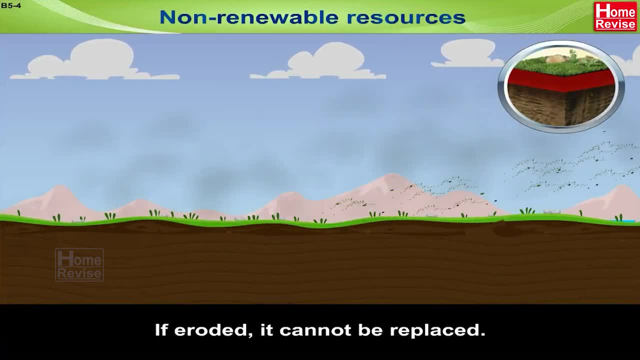 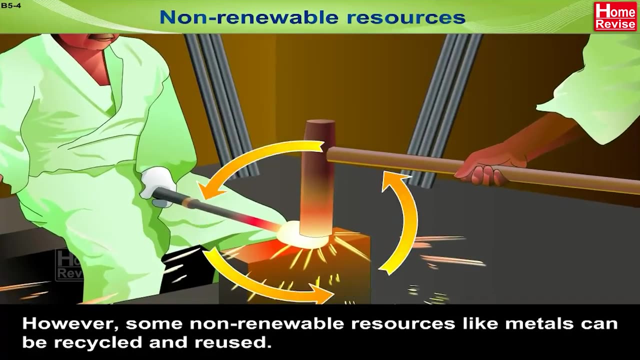 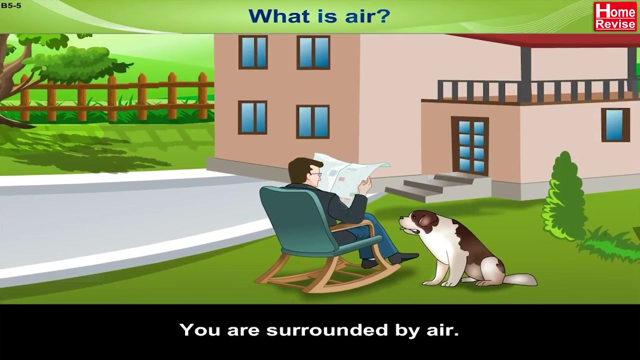 Similarly, it takes hundreds of years for a few centimetres of topsoil to form. If eroded, it cannot be replaced. However, some non-renewable resources, like metals, can be recycled and reused. What is air? You are surrounded by air. 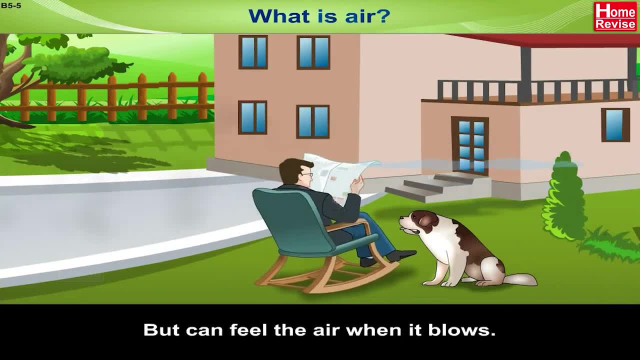 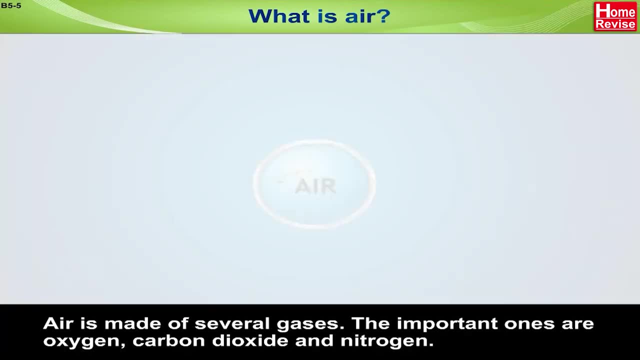 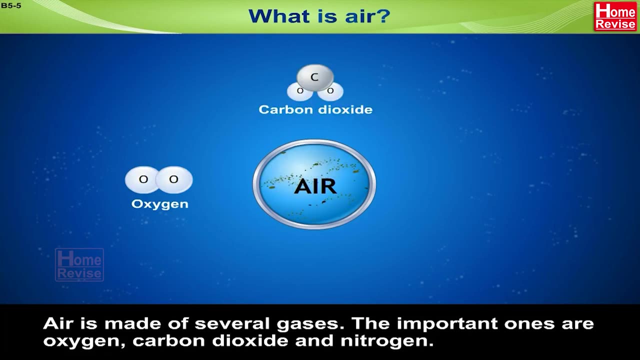 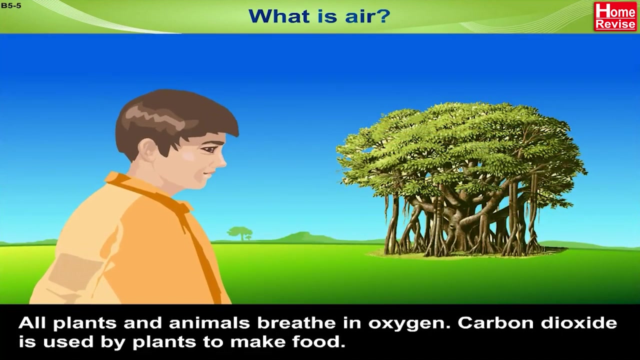 You cannot see it, but you can feel the air when it blows. Moving air is called wind. Air is made of several gases. The important ones are oxygen, carbon dioxide and nitrogen. All plants and animals breathe in oxygen. Carbon dioxide is used by plants to make food. 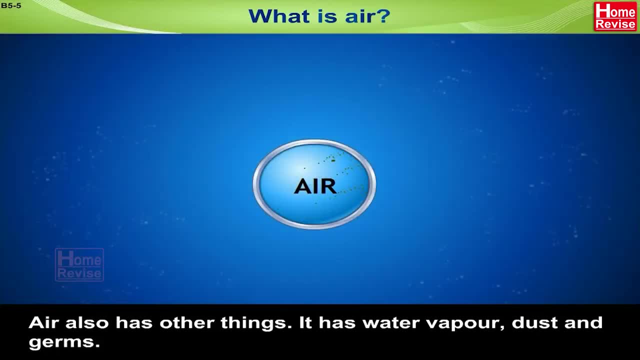 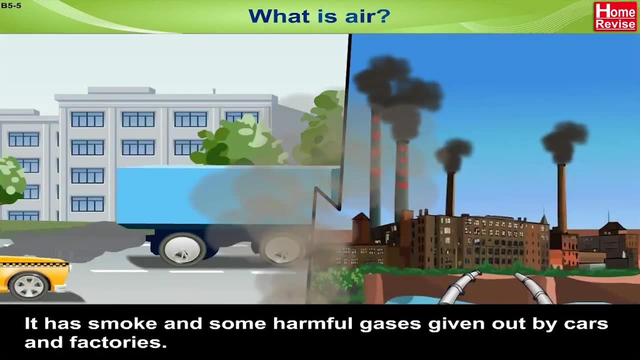 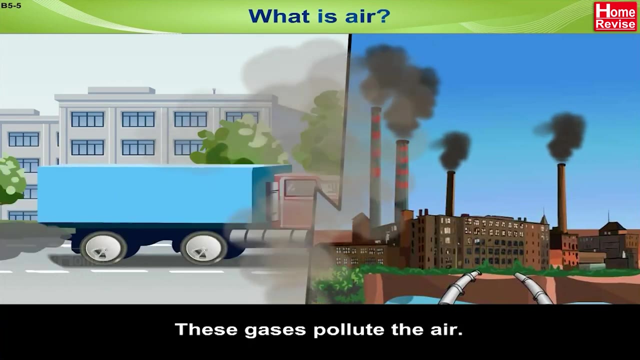 Air also has other things. It has water, vapour, dust and germs. It has smoke and some harmful gases given out by cars and factories. These gases pollute the air. When you breathe in this polluted air, you can get sick. 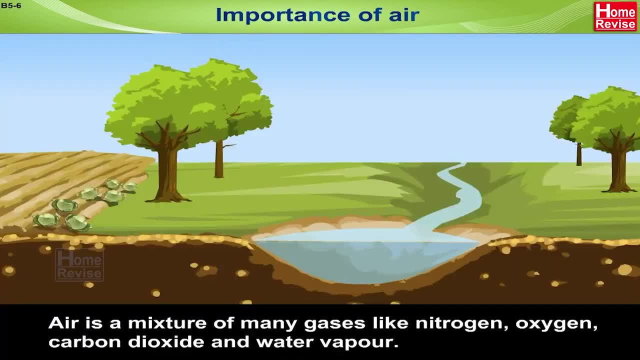 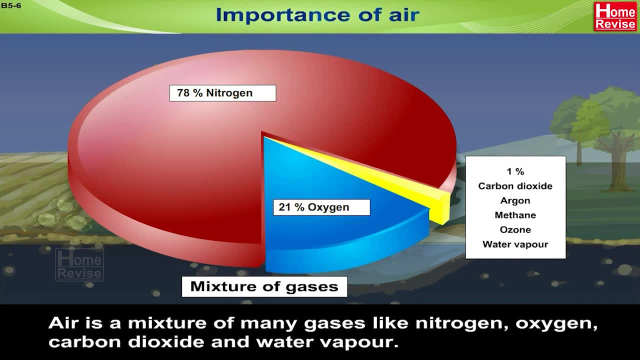 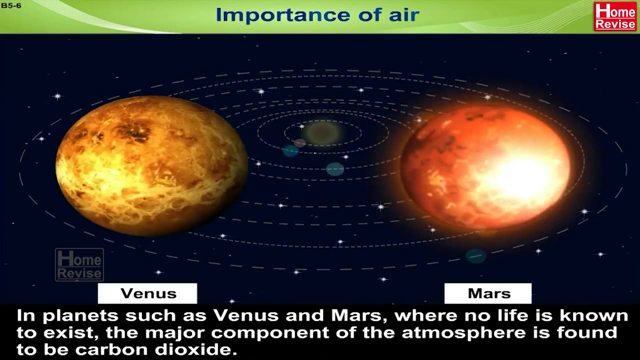 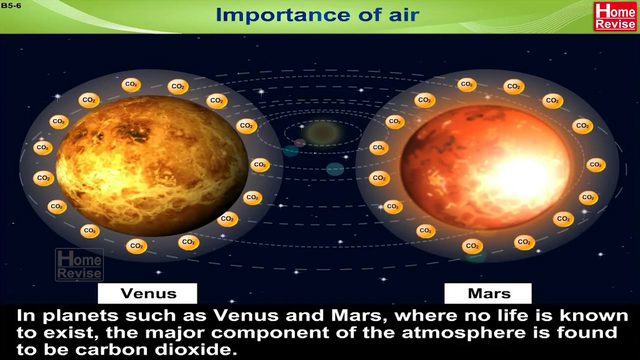 Air is a mixture of many gases like nitrogen oxygen, carbon dioxide and water vapour. In planets such as Venus and Mars, where no life is known to exist, the major component of the atmosphere is found to be carbon dioxide. In fact, carbon dioxide is the main component of the atmosphere. 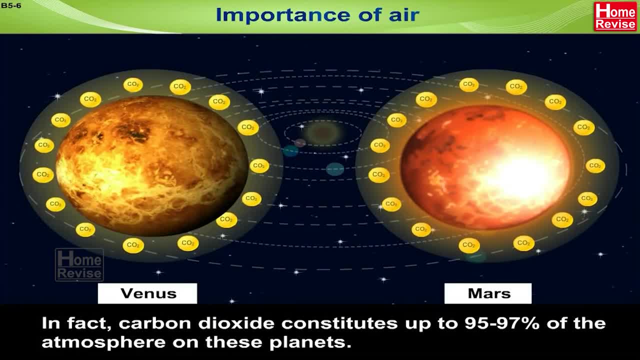 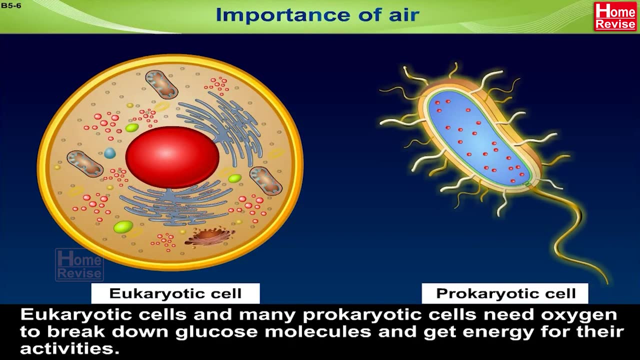 It is the main component of the atmosphere. In fact, carbon dioxide is the main component of the atmosphere. In fact, carbon dioxide constitutes up to ninety five to ninety seven percent of the atmosphere on these planets. Eukaryotic cells and many prokaryotic cells need oxygen to break down glucose molecules. 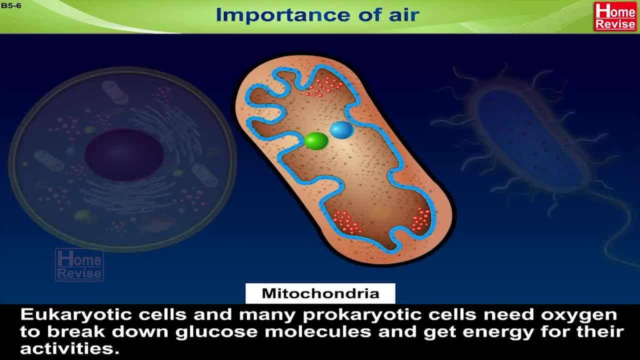 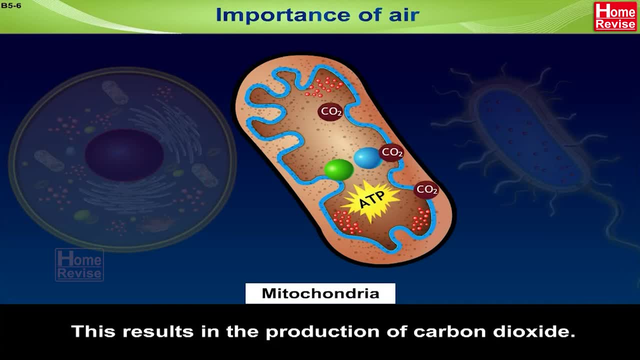 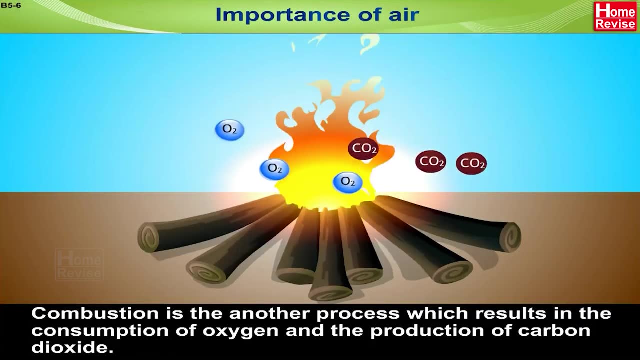 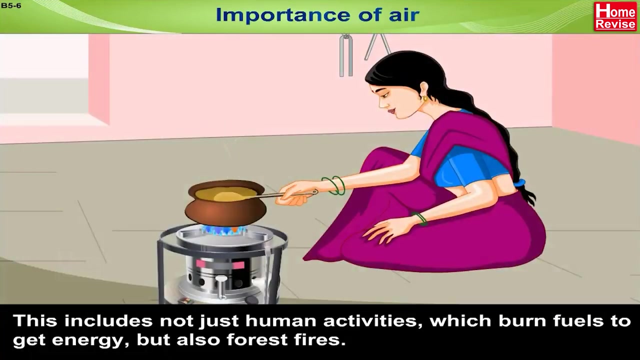 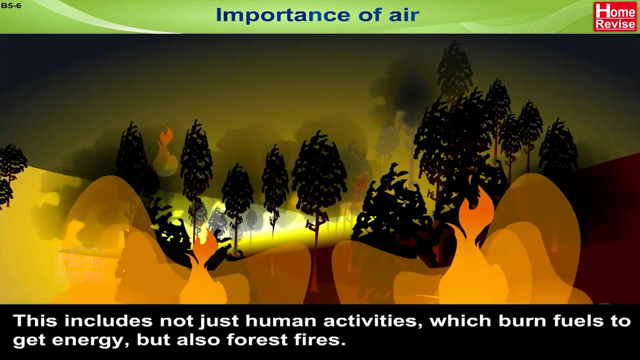 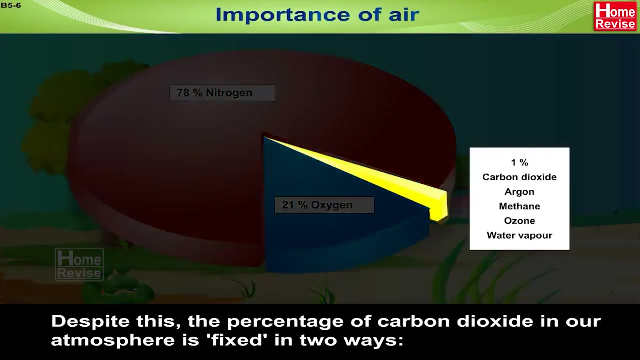 and get energy for their activities. This results in the production of carbon dioxide. Combustion is another process which results in the consumption of oxygen and the production of carbon dioxide. This includes not just human activities which burn fuels to get energy, but also forest fires. Despite this, the percentage of carbon dioxide in our atmosphere is fixed. 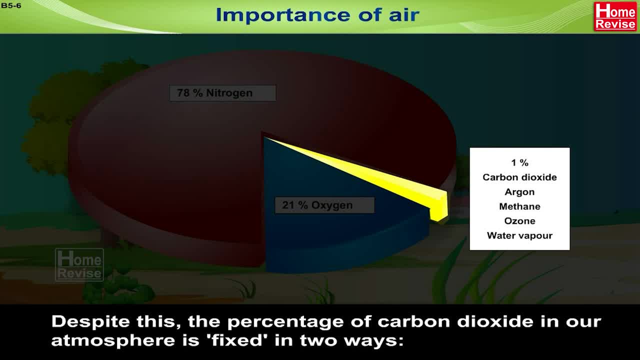 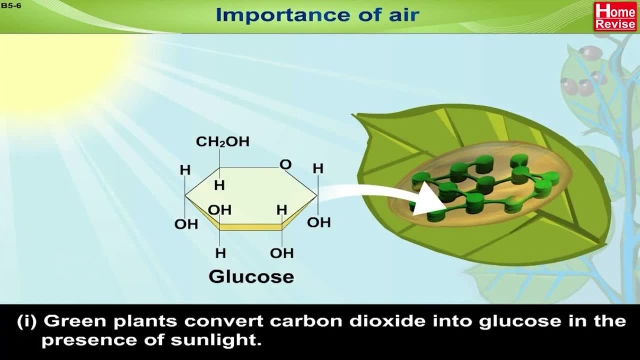 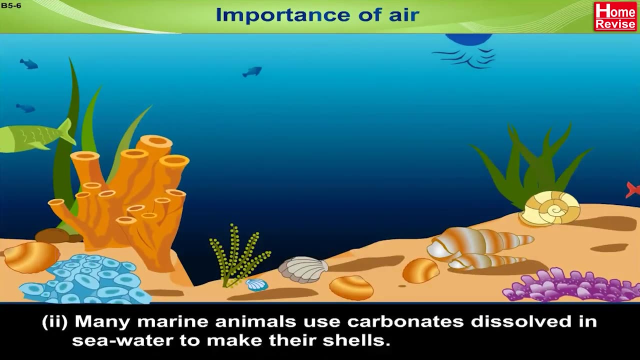 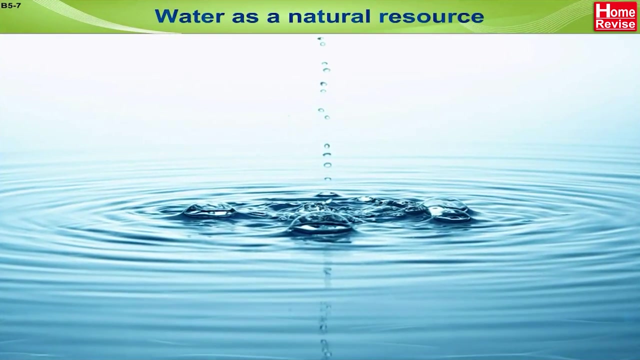 in two ways: Green plants convert carbon dioxide into glucose in the presence of sunlight, and many marine animals use carbonate to burn fuel. Carbon dioxide is a massive energy container which is interested in the superconductivity of the earth's ultraviolet rays. The superconductivity of carbon dioxide is higher than that of any. 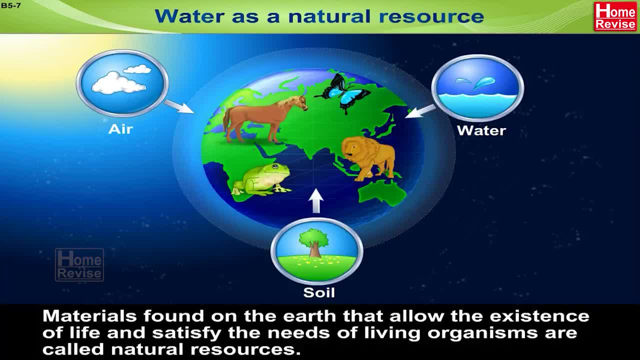 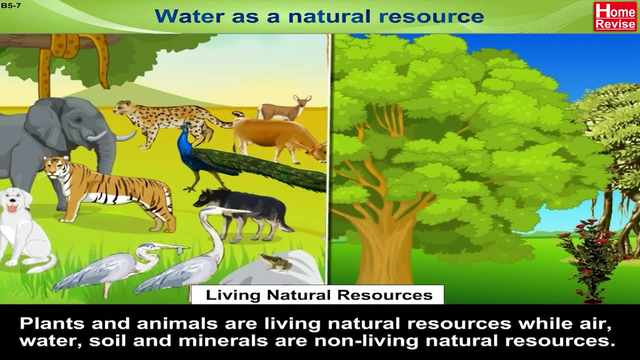 organic matter. Calcium is also a massive energy generator and it will transport a large amount of oxygen which will transfer further into our atmosphere. 5. Water: Water is a natural resource. Let us know in the comments below if you have any questions. 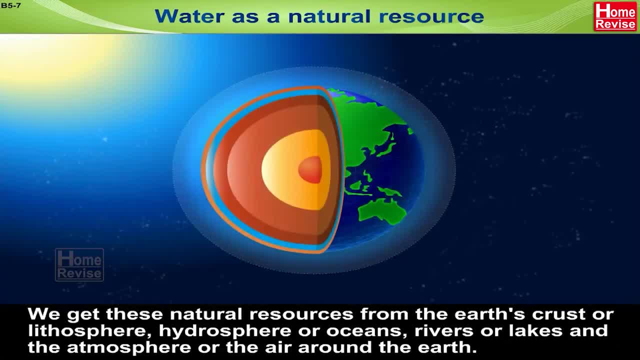 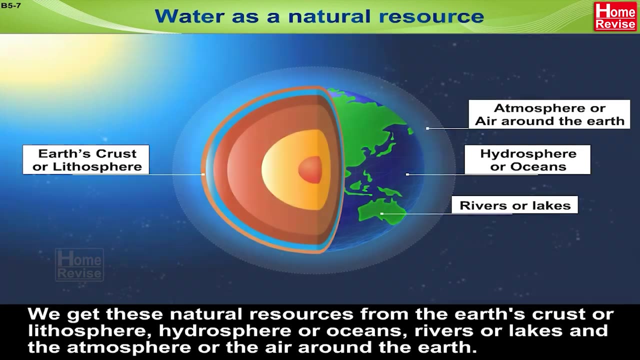 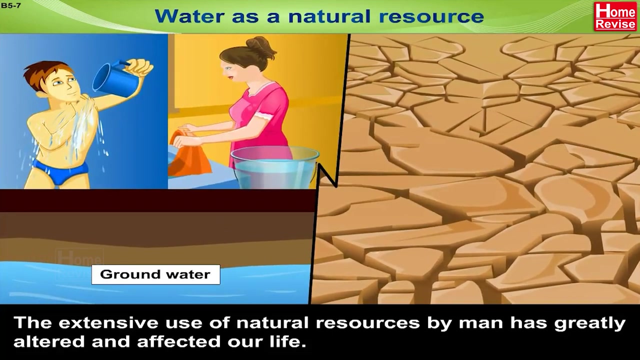 resources. We get these natural resources from the earth's crust or lithosphere, hydrosphere or oceans, rivers or lakes, and the atmosphere or the air around the earth. The extensive use of natural resources by man has greatly altered and affected our life. 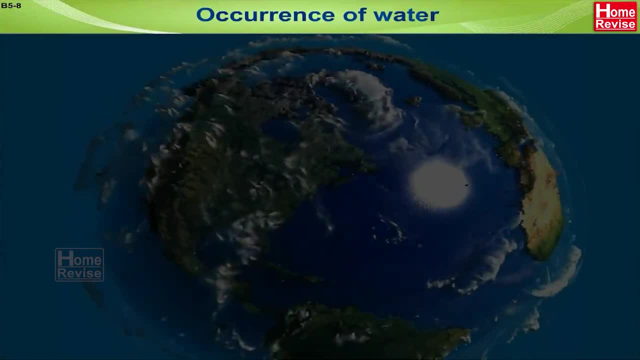 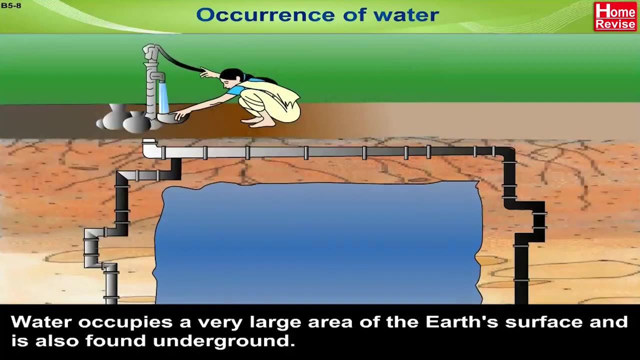 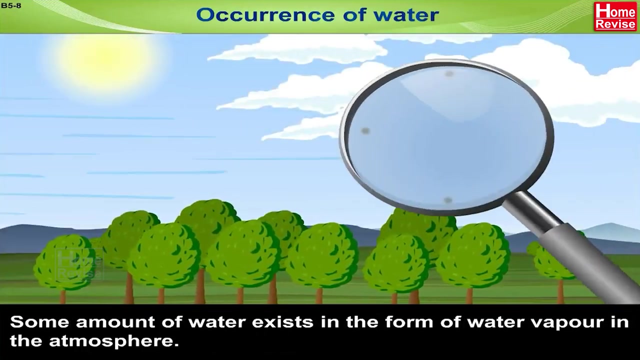 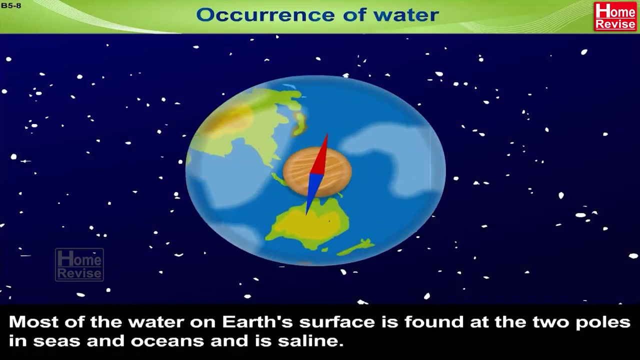 OCCURRENCE OF WATER. Water occupies a very large area of the earth's surface and is also found underground. Some amount of water exists in the form of water vapour in the atmosphere. Most of the water on earth's surface is found at the two poles. 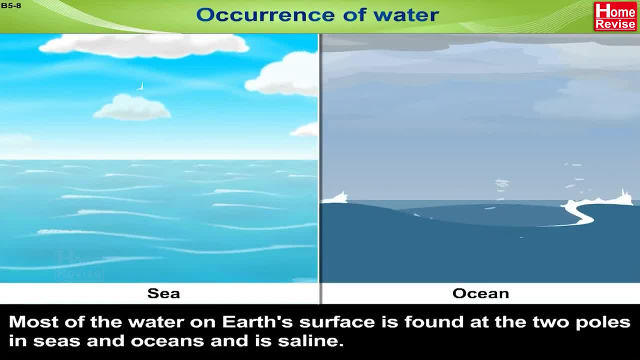 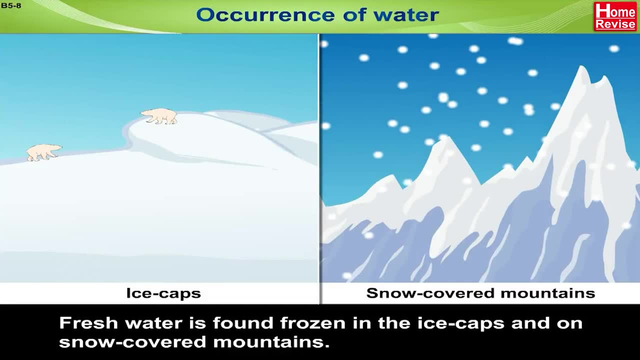 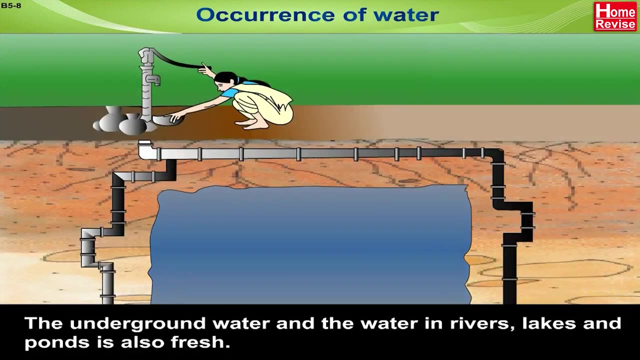 in seas and oceans or in the atmosphere. Most of the water on earth's surface is found in the ice caps and is saline. Fresh water is found frozen in the ice caps and on snow covered mountains. The underground water and the water in rivers, lakes and ponds is also. 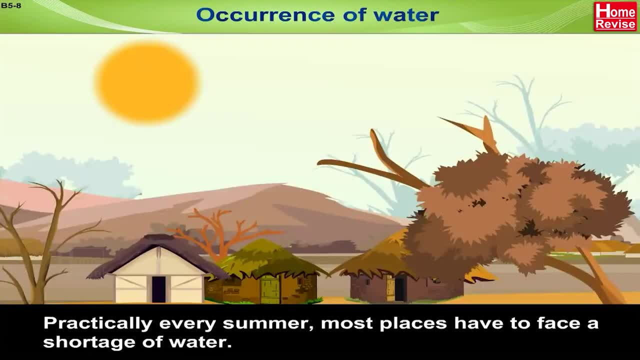 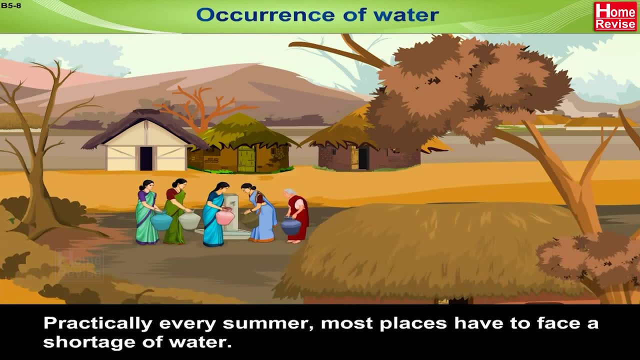 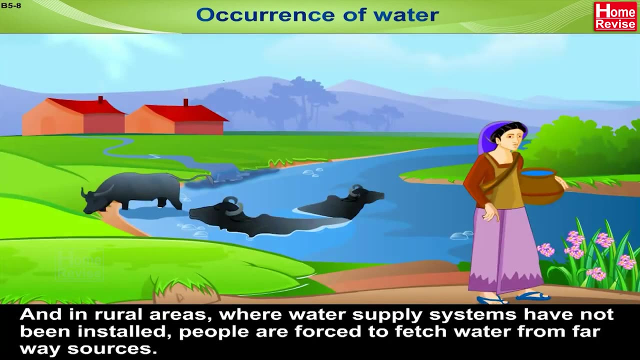 fresh. Practically every summer, most places have to face a shortage of water. We are all familiar with water shortage in summers, aren't we? And in rural areas where water supply systems have not been installed, people are forced to fetch water from far away sources. Quite tedious it is actually. 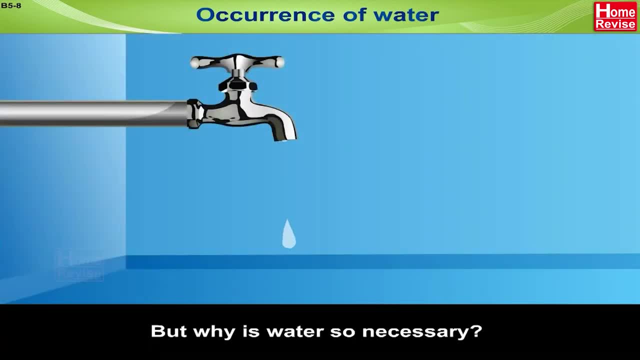 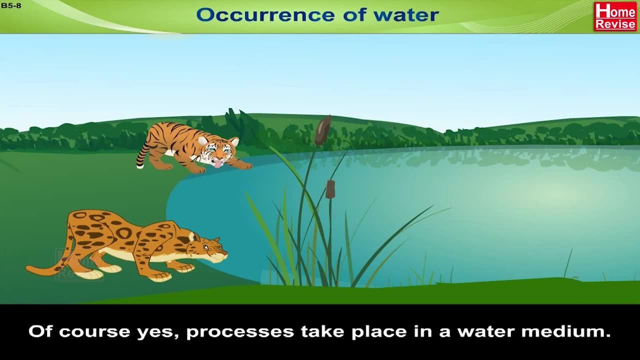 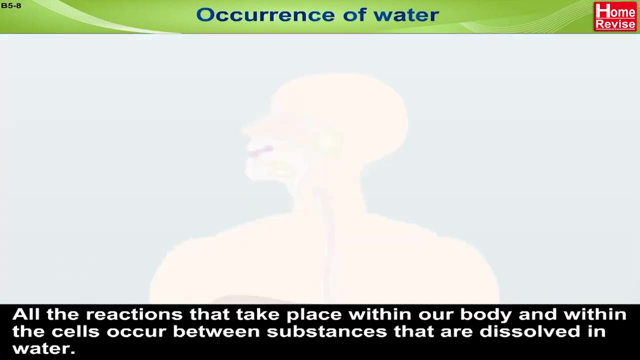 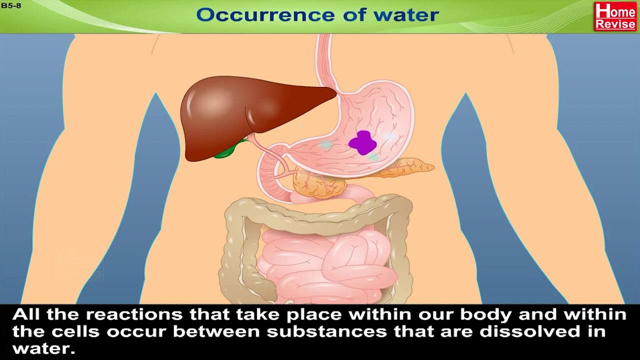 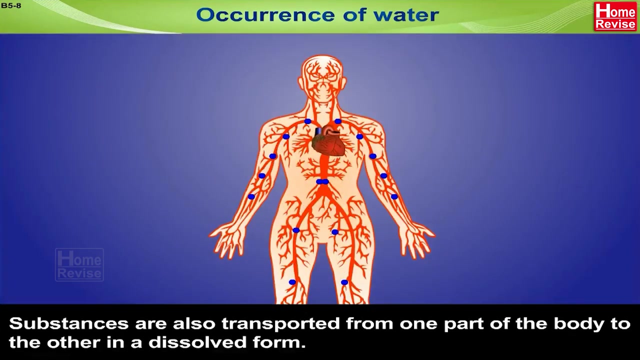 But why is water so necessary, And do all organisms require water? Of course yes. Processes take place in a water medium. All the reactions that take place within our body and within the cells occur between substances that are dissolved in water. Substances are also transported from one part of the body to the other in 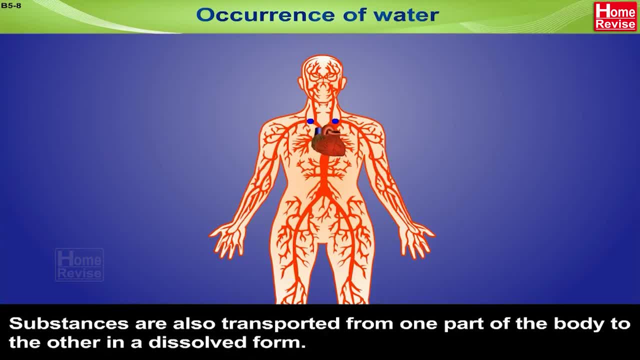 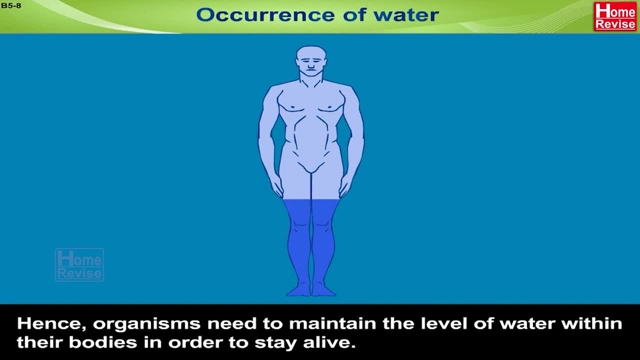 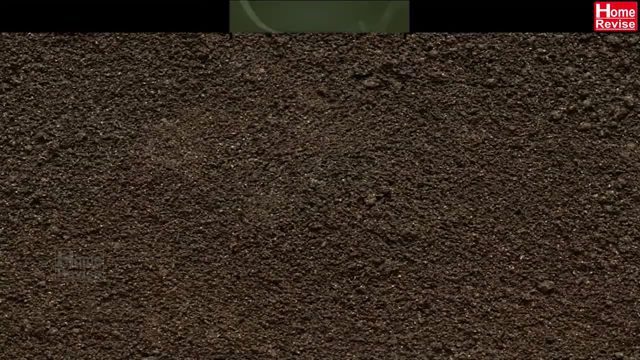 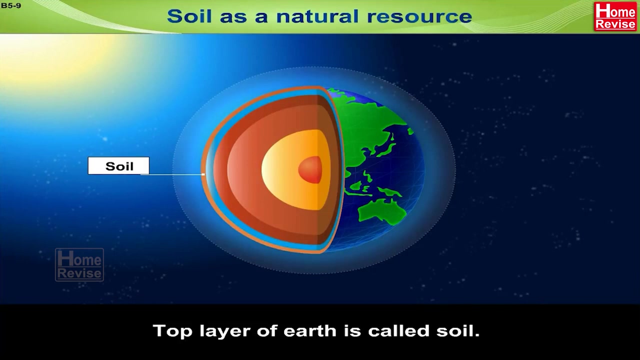 a dissolved form. Hence organisms need to maintain the level of water within their bodies in order to stay alive. That's how important water is to all of us. Soil as a Natural Resource. Top layer of earth is called soil. It is the main natural resource required for survival. 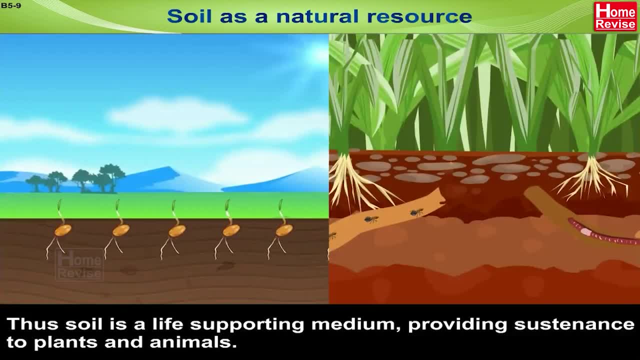 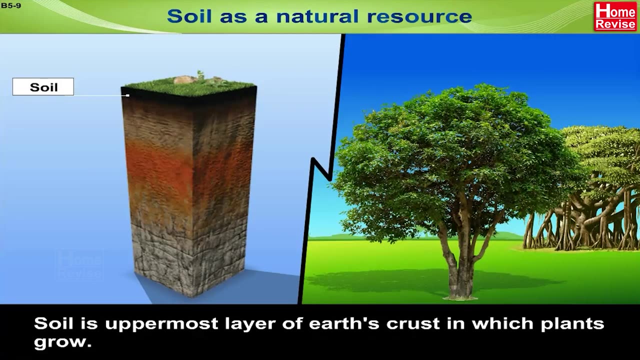 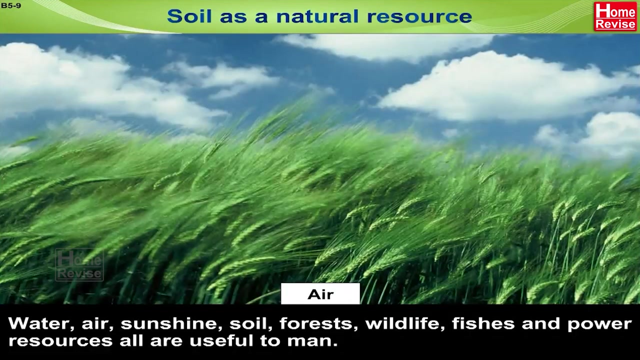 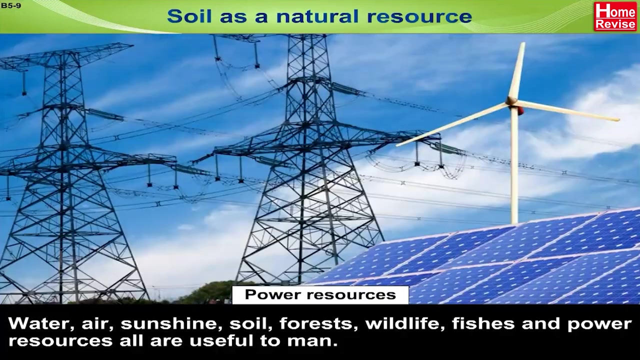 of living beings. Thus, Soil is a supporting medium providing sustenance to plants and animals. soil is the uppermost layer of Earth's crust in which plants grow. a natural resource satisfies human wants: water, air, sunshine, soil, forests, wildlife, fishes and power resources- all are useful to man. more than four-fifths of